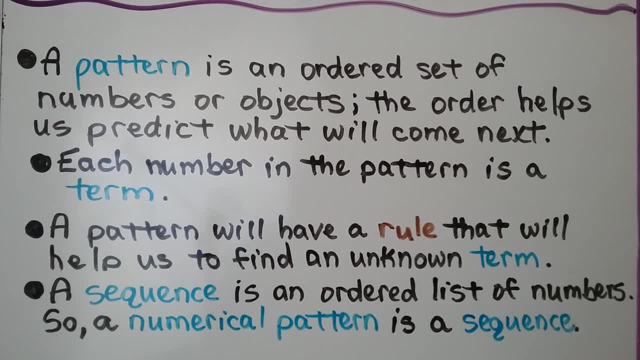 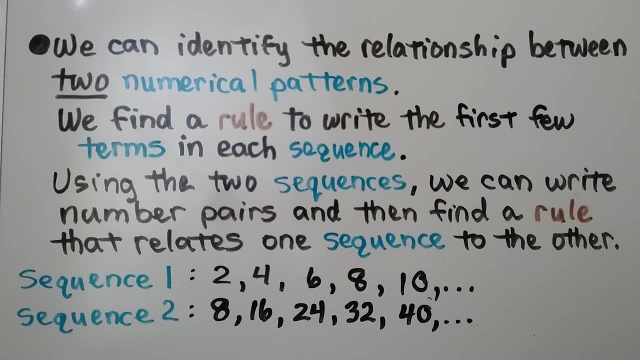 so a numerical pattern is a sequence. We can identify the relationship between two numerical patterns. We find a rule to write the first few terms in each sequence. Using the two sequences, we can write number pairs and then find a rule that relates one sequence to the other. We have 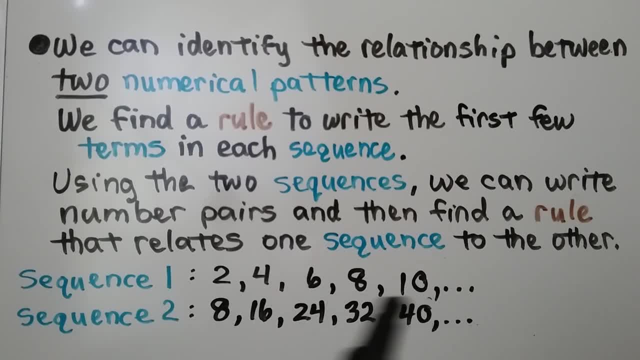 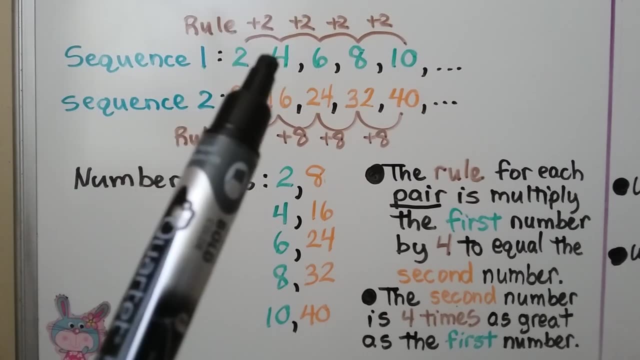 sequence one, it's got two, four, six, eight, ten and sequence two has eight, sixteen, twenty-four, thirty two. The rule for sequence one is: add two. We go from two to a four. We added two. We add two more. We get to six. We add two more We. 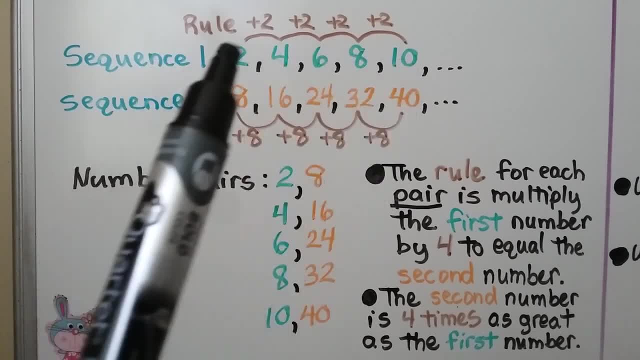 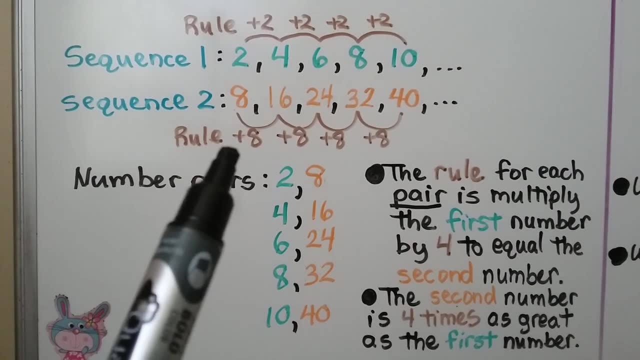 get to eight, We add two more, We get to ten. So the rule for this sequence is to add two. We know the next number would be twelve. For sequence two, the rule is add eight to get to the next one term in the sequence. We can write them as number pairs, the 2 and the 8, as a 2, 8, the 4 and 16. 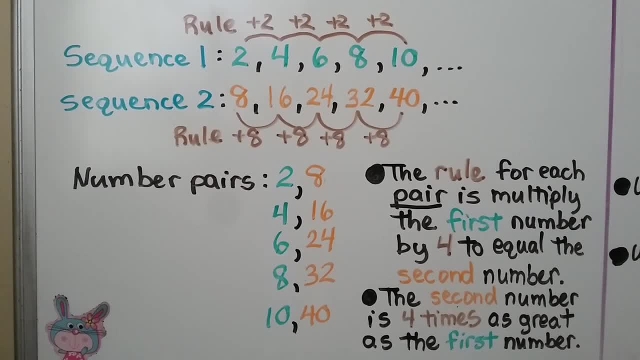 as a 4,, 16, and so on. And the rule for each pair is: multiply the first number by 4 to equal the second number. If we multiply 2 times 4,, it will be 8.. If we multiply 4 times 4,, it'll be 16,. 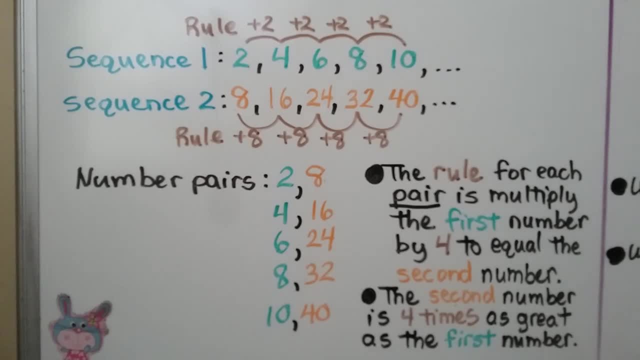 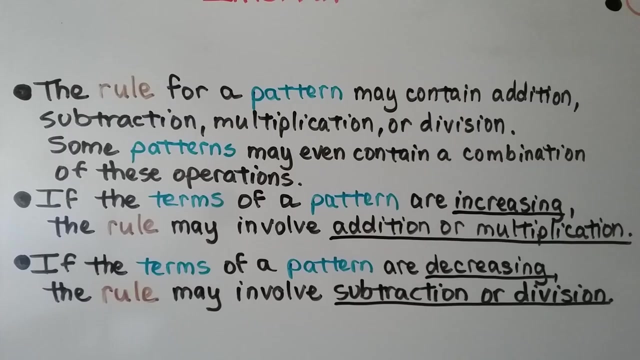 and 6 times 4 is 24.. The second number is 4 times as great as the first number. The rule that relates sequence 1 to sequence 2 is multiply by 4.. The rule for a pattern may contain addition, subtraction, multiplication or division. Some patterns may even contain a combination of these. 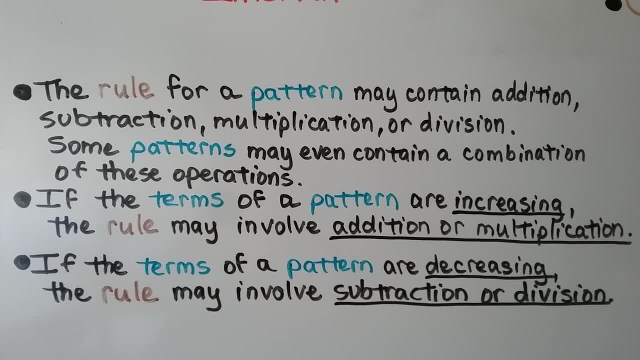 operations. If the terms of a pattern are incorrect, the rule for a pattern may contain a combination of these operations. If the terms of a pattern are incorrect, the rule for a pattern are increasing. the rule may involve addition or multiplication, And if the terms of a pattern are. 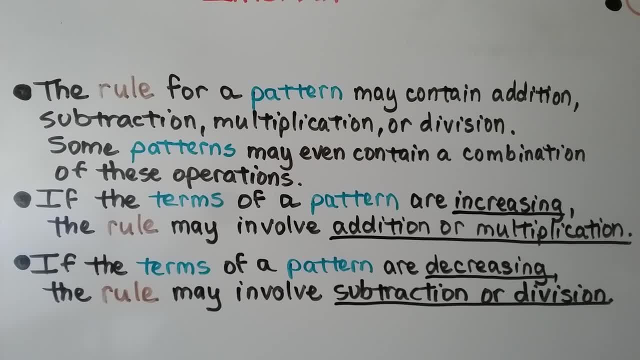 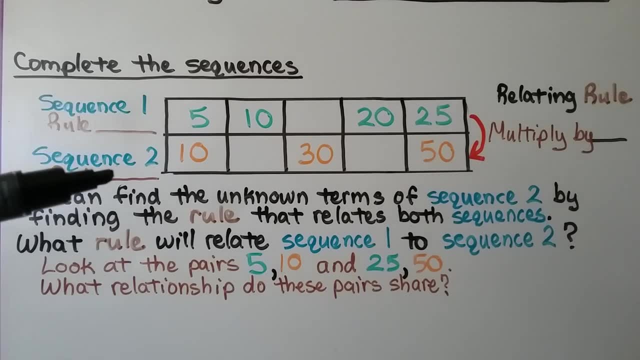 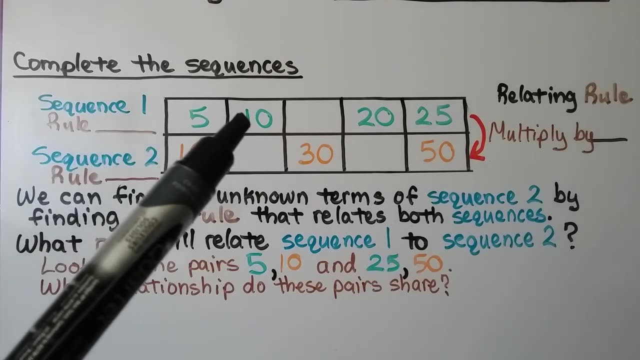 decreasing the rule may involve subtraction or division. We need to complete the sequences here. We need to find the rule for each sequence. For sequence 1, it's going from 5 to 10, then we have a missing term and then it took from 20 to 25.. To go from 15,: 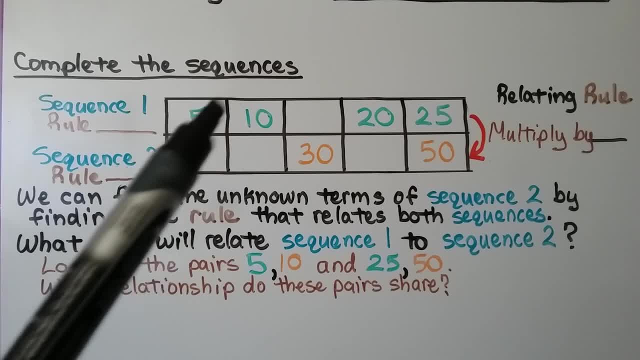 to 25, to 10, we have to find the rule for each sequence. For sequence 1, we have to go from 5 to to 10, we need to add 5 or multiply by 2. but to go from 20 to 25, we need to add. 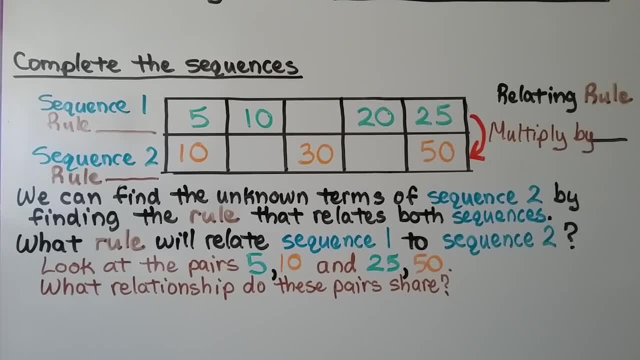 5. so we know multiply by 2 is not the rule, otherwise this would go from 20 to 40. it must be add 5. if the rule is to add 5, we know the missing term must be 10 plus 5. it must be 15. we have a missing term here in sequence 2 and 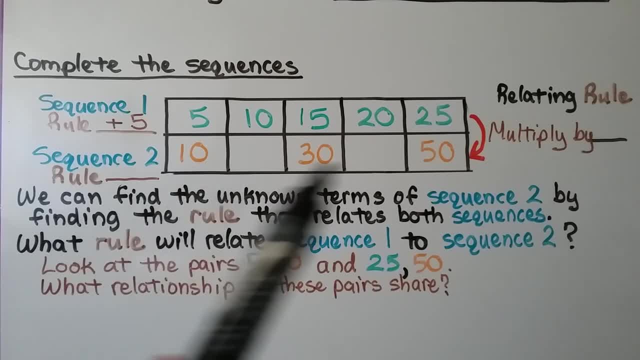 another missing term. we don't have enough information to finish this or to write its rule, but we can find the unknown terms of sequence 2 by finding the rule that relates both sequences. we find a rule that relates sequence 1 to sequence 2 and we can look at the pairs 5 and 10. 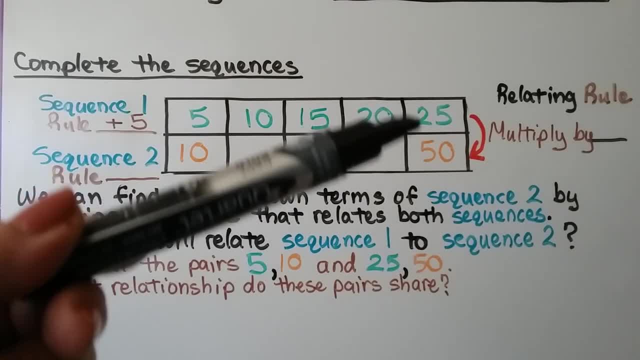 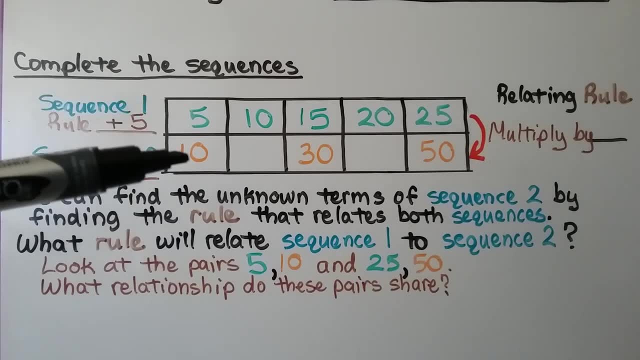 and we can look at the pairs 5 and 10, and we can look at the pairs 5 and 10 and we can even look at 15 and 30 and 25 and 50. what relationship do these pairs share? what do we need to do to the 5 to make it a 10? what do we need to do to 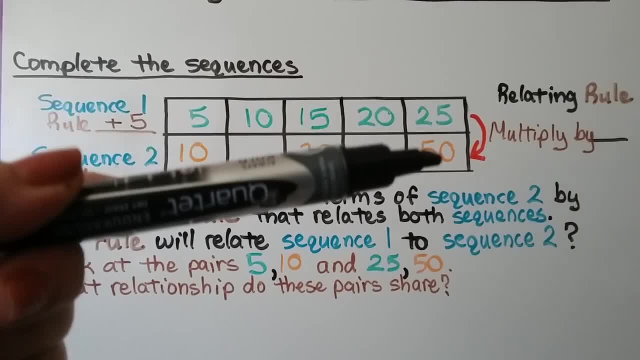 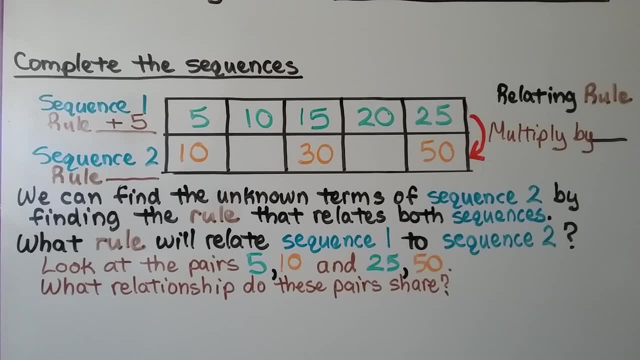 the 15 to make it a 30, and what do we need to do to the 25 to make it a 50? if you said multiply by 2, you're right. the rule that relates sequence 1 to sequence 2 is multiplied by 2. that means that the rule that relates sequence 1 to 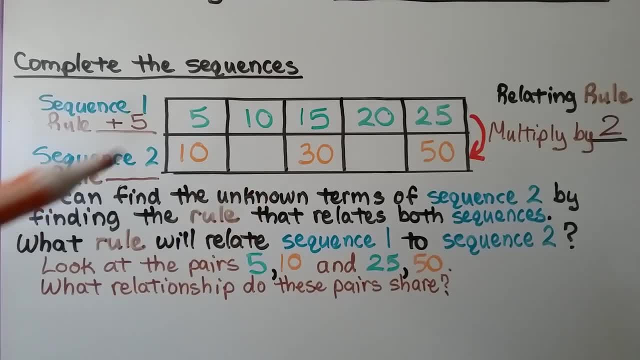 sequence 1 and sequence 2 is multiplied by 10, is the 20th step. it'll be Zeke's sovereignty law that noodles 5, 11 and 5, now that we have Isso, multiply by 2.. Let's try it again with this one. Let's complete the sequences. 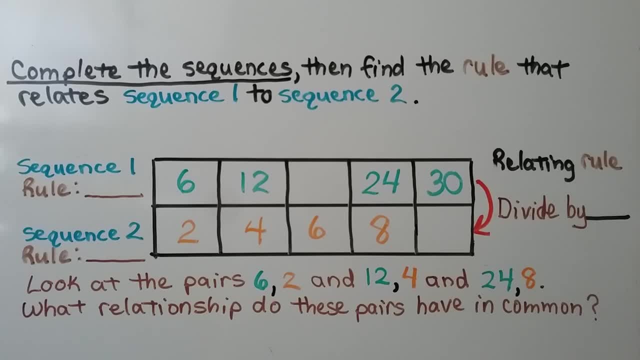 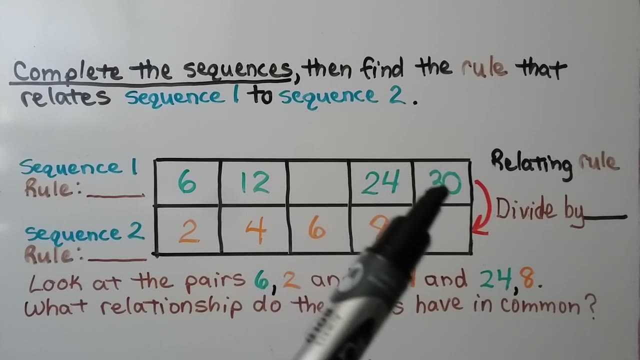 then find the rule that relates sequence 1 to sequence 2. We look at the relationship between 6 and 12. Well, that could be 6 times 2, but it could also be 6 plus 6. We don't have this term, and 24 plus 6 is 30, so we know it's not times. 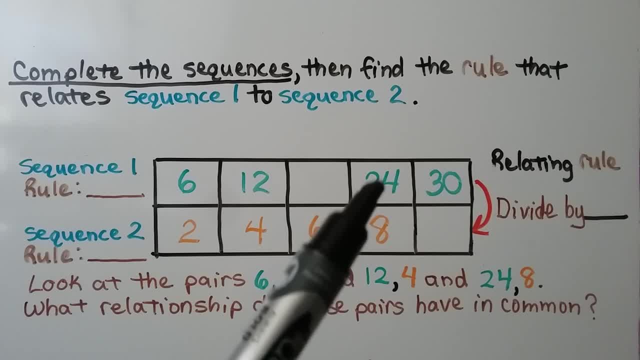 2, because if it was times 2,, 24 times 2 would be 48, and that's only a 30. So we know the rule is plus 6 for sequence 1.. If it's plus 6, we know the missing term. 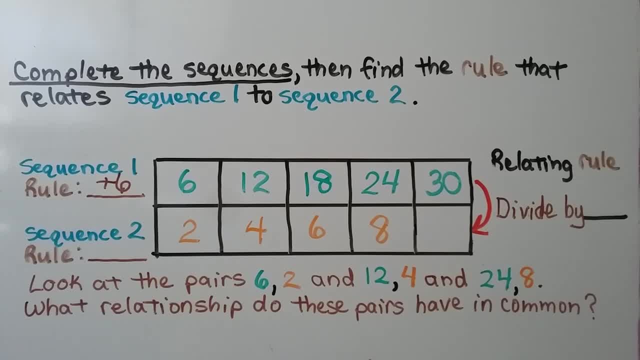 is 18.. We can look at the sequence of numbers, the terms in sequence 2, it's going 2, 4, 6, 8.. This rule is plus 2.. If the rule is plus 2, we know that this term must be 10.. We need to find the rule. 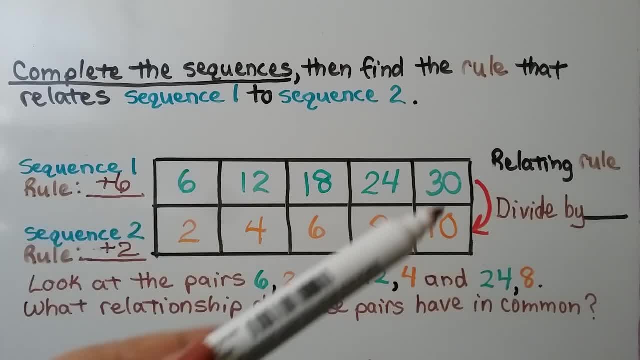 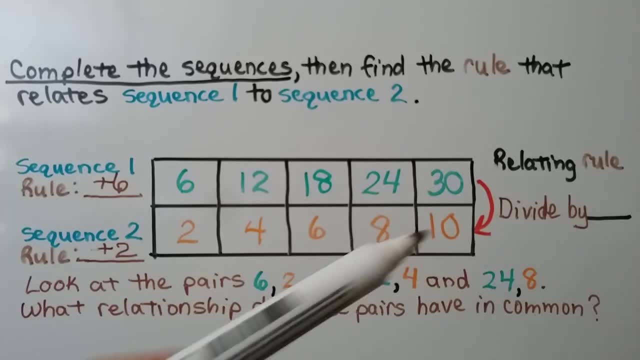 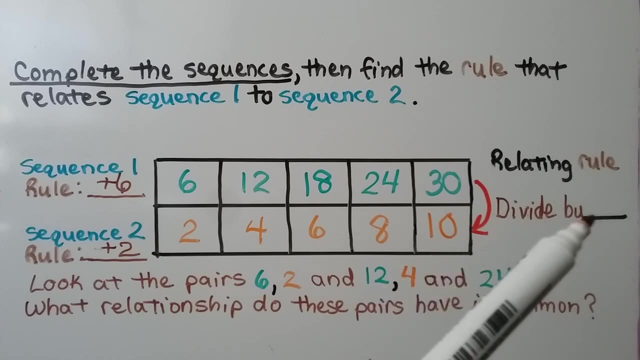 that relates sequence 1 to sequence 2.. Notice the arrow and the direction the arrow is going in. It's going from 30 to 10.. That means, because it's decreasing, we're going to subtract or divide and it tells us: divide by 30,. 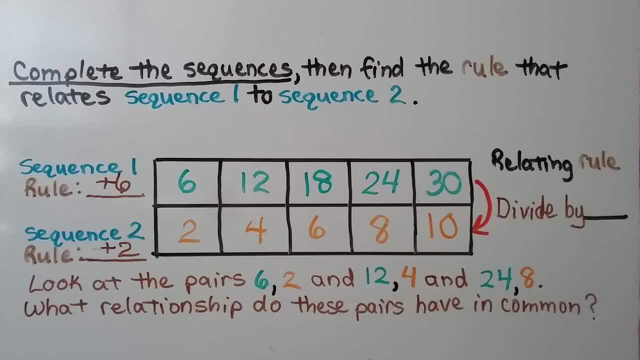 divide by 30, by 3 is equal to 10.. We check the other terms: 24 divided by 3 is 8,, 18 divided by 3 is 6,, 12 divided by 3 is 4, and 6 divided by 3 is 2.. We look at the pairs. 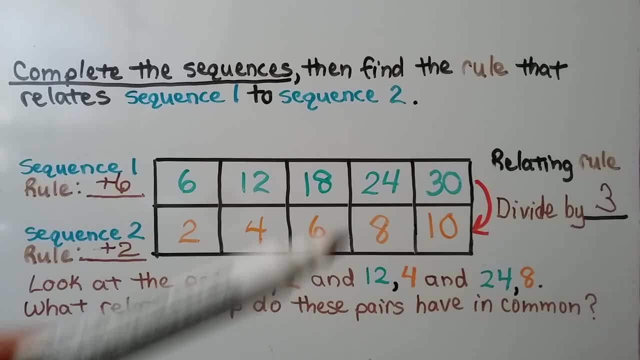 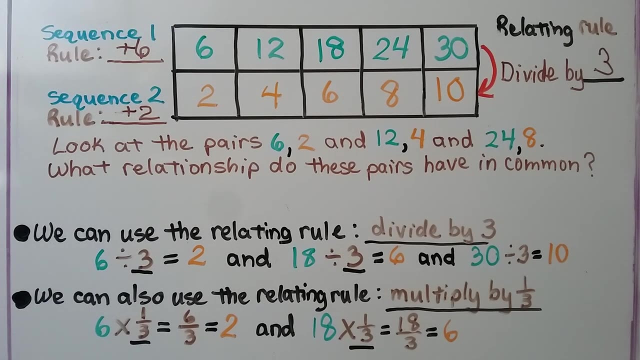 of 6, 2 and 12, 4 and all of them, and look at the relationship that these pairs have in common, So we can use the relating rule: divide by 3.. 6 divided by 3 is equal to 2 and 18 divided by 3 is equal to 6, and 30 divided by 3 is equal. 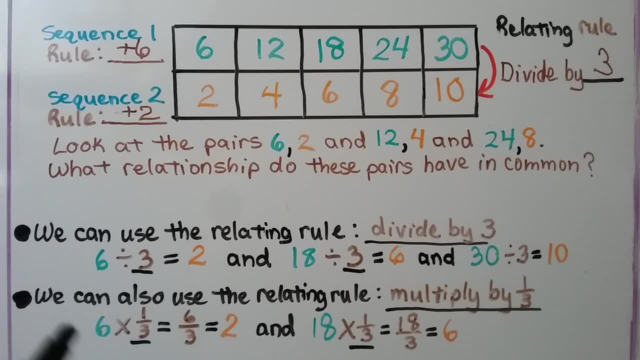 to 10.. But we can also use the relating rule: multiply by 1- 3rd, 6 times 1 3rd is equal to 6 3rds, which simplifies to 2, and 18 times 1- 3rd is equal to 18 3rds, which simplifies to 6.. So we could use the 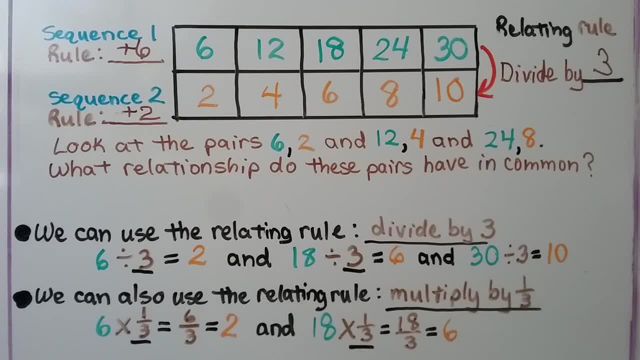 rule: divide by 3 or multiply by 1. 3rd, We look at the direction that the arrow is heading. We know that this is going to be the first number like this is a 6, and we know that it's going to equal this number. 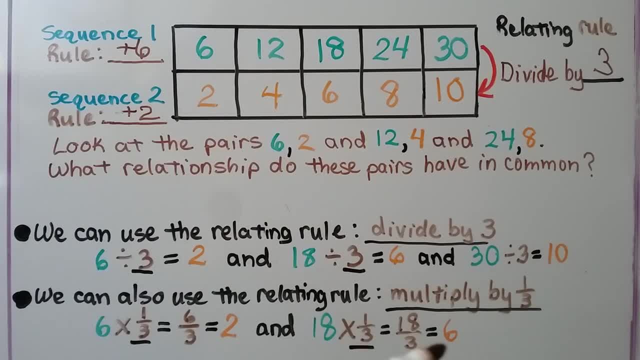 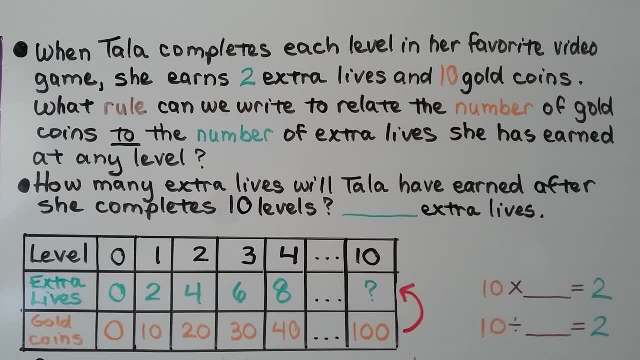 18 is the first number and it's going to equal 6.. When Tala completes each level in her favorite video game, she earns 2 extra lives and 10 gold coins. What rule can we write to relate the number of gold coins to the number of extra lives? 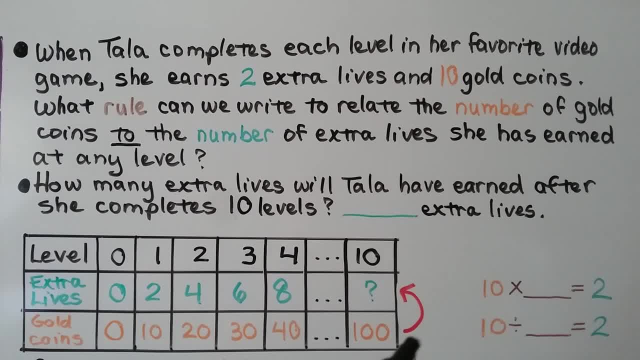 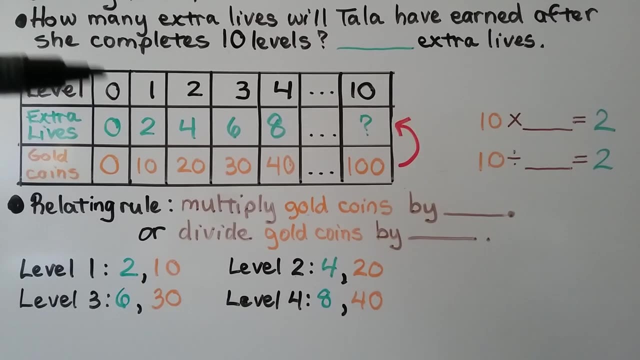 that she has earned at any level. Notice the arrow is now going up towards the extra lives. So how many extra lives will Tala have earned after she completes 10 levels? We compare the values for the extra lives and gold coins to each other. 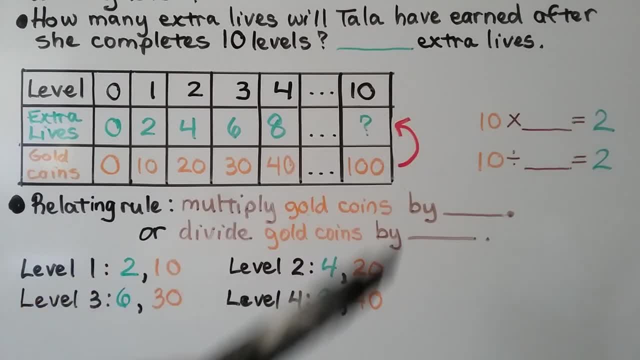 starting with gold coins, because the arrow is going upward. 10 became a 2.. What would we have to do to 10 to make it a 2?? We could divide it by 5.. But what could we multiply all the extra gold coins by so that it would equal the extra lives? 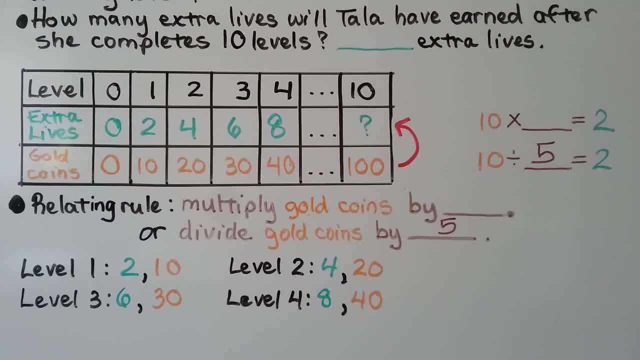 If you said multiply it by one-fifth, you are right. 10 x one-fifth would be 10 Cube Pits. that would simplify to two. We can multiply the gold coins by one-fifth or divide the gold coins by 5.. 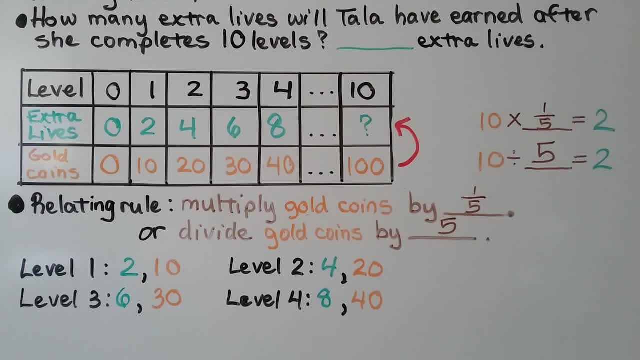 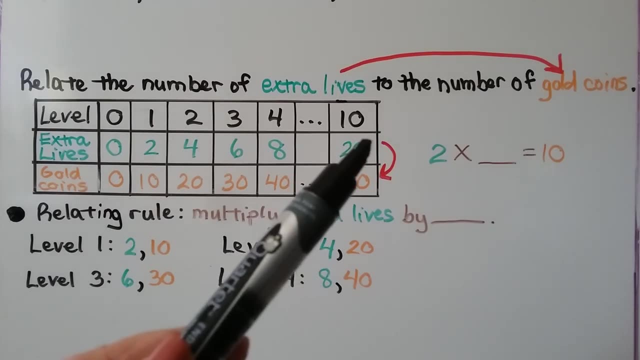 100! divided by 5 would be equal to do you know? that would be 20.. She'd have 20 extra lives If the arrow is going down to the 100, in the last one it was going up towards the 20,. 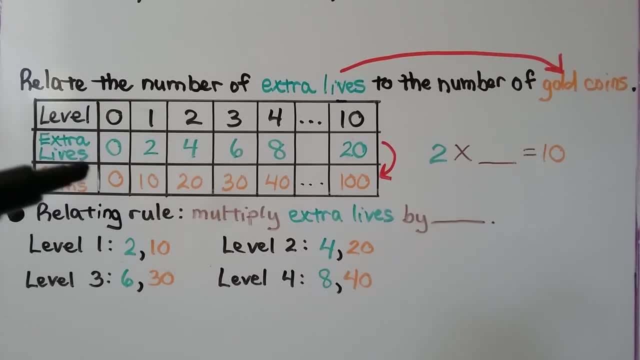 we can relate the number of extra lives to the number of gold coins. Before we did multiplying the amount of gold coins by some amount to equal the extra lives. Now we're going to start with extra lives as our first number. We're going to multiply it by some amount to equal 10.. 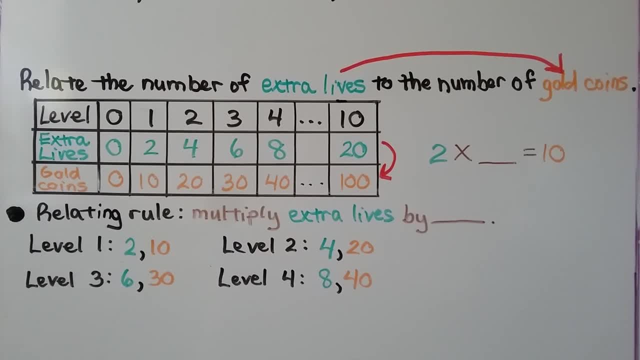 If you said 5, you're right. We can look at the number pairs. It goes from 2 to 10, and 2 times 5 is 10.. For this one, 4 times 5 is 20,, 6 times 5 is 30, and 8 times 5 is 40.. 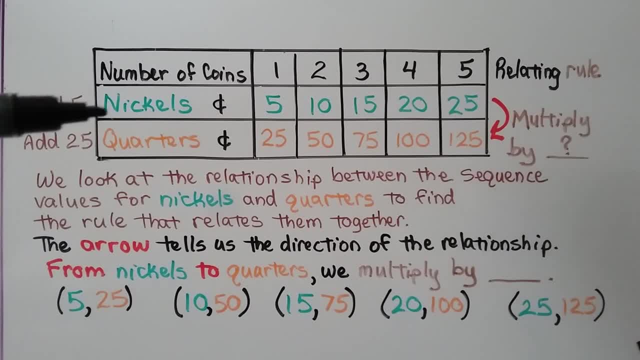 Here we have number of coins, we have nickels, we have quarters, and it's telling us that the rule for the nickels is to add 5.. If we have 1 nickel, we have 5 cents. If we have 2 nickels, we have 10 cents. 3 nickels is 15 cents, and so on. For quarters, we add: 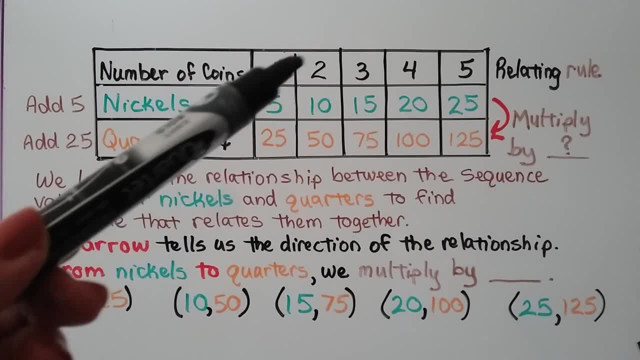 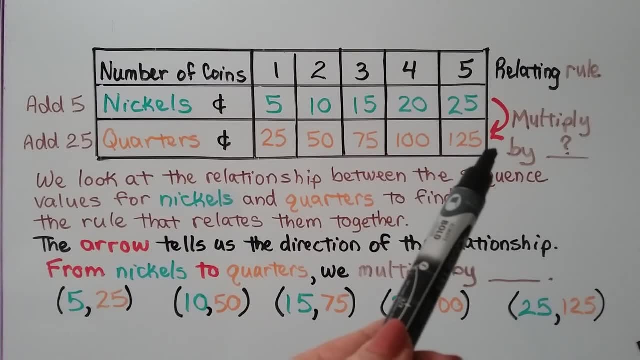 25.. For 1 quarter, we have 25 cents. for 2 quarters, we have 50 cents. for 3 quarters, we have 75 cents, and so on. We look at the arrow. The arrow is going from the nickels to 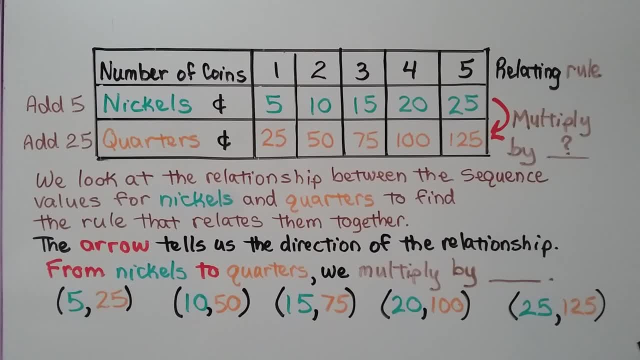 the quarters. We look at the relationship between the sequence values for nickels and quarters to find the rule that relates them together. The arrow tells us the direction of the relationship. It's going from nickels to quarters, to go from a 5 to a 25, do you know what? we would need to multiply by Or to go. 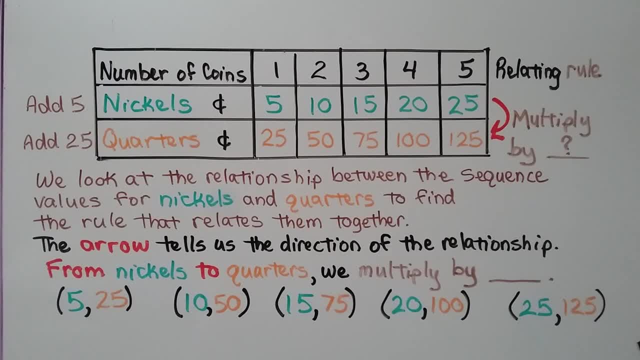 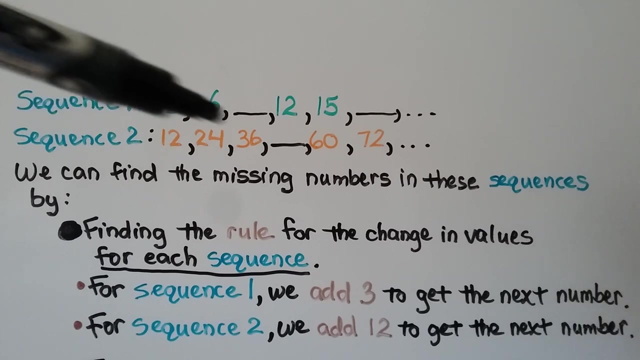 from a 10 to a 50?. If you said multiply by 5, you're right. The rule that relates the sequence of nickels to the sequence of quarters is multiply by 5.. Here we have sequence 1, and it's missing two terms. Here we have sequence 2, and it's. 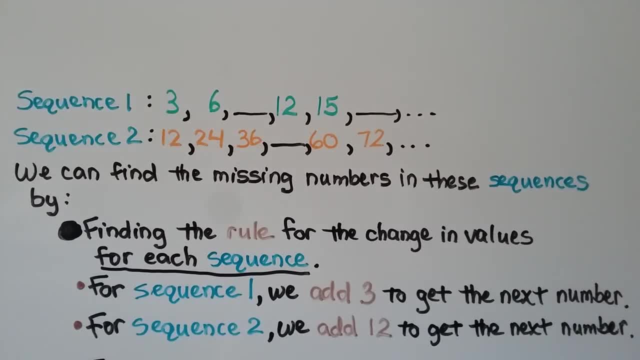 missing one term. We can find the missing numbers in these sequences by finding the rule for the change in values for each sequence. For sequence 1, we add 3 to get the next number, And for sequence 2, we add 12 to get the next number. So 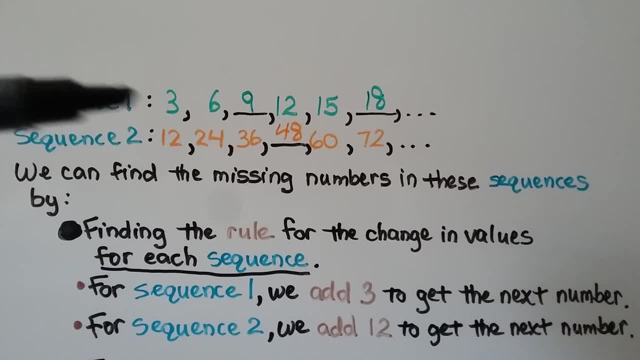 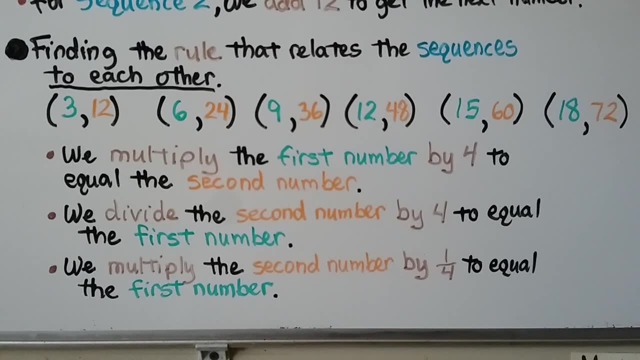 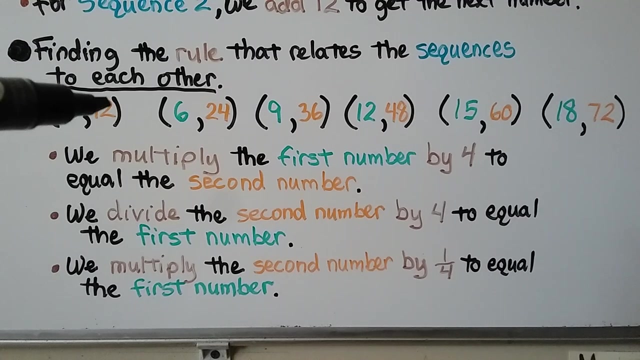 by finding each of their separate rules, we can complete the sequences and fill in the unknown terms. We can find the missing numbers in the sequences by finding the rule that relates the sequences to each other. We have a 3 and a 12, a 6 and a 24.. We multiply the first number by 4 to get the second number. 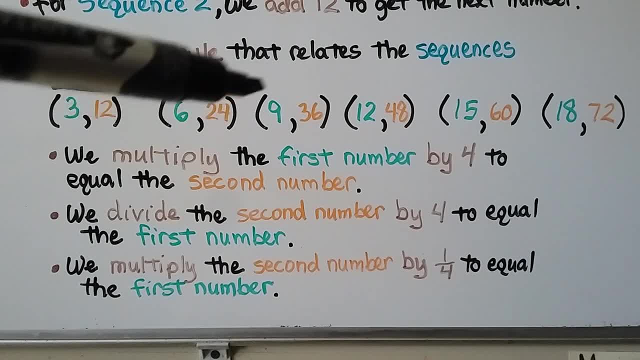 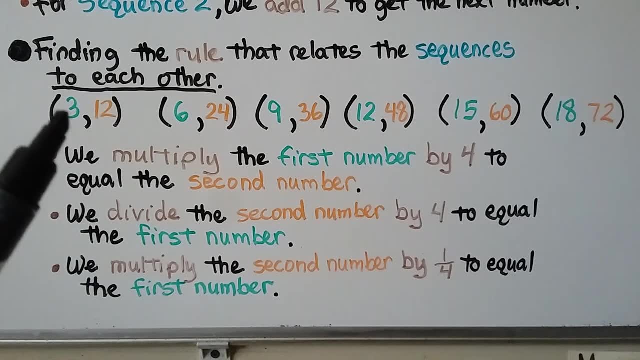 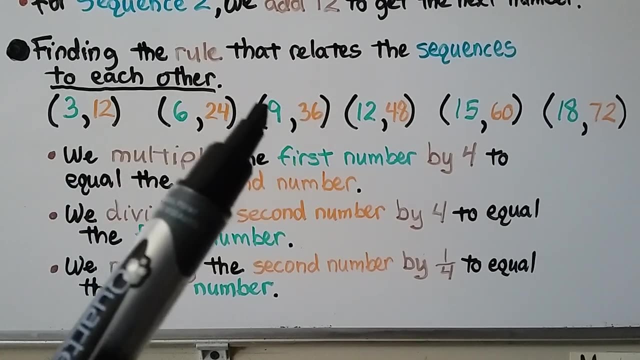 3 times 4 is 12.. 6 times 4 is 24.. 9 times 4 is 36.. We could also divide the second number by 4 to equal the first number. 12 divided by 4 is 3,. 24 divided by 4 is 6,. 36 divided by 4 is 9.. We could also: 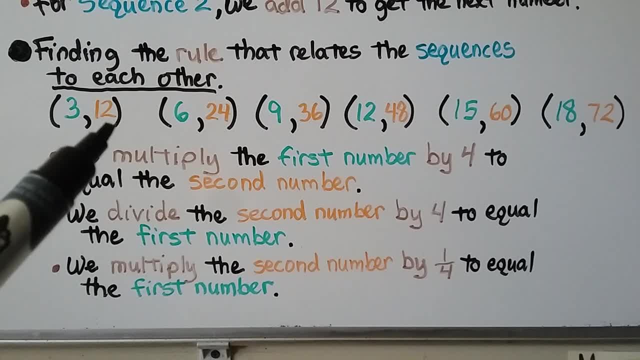 multiply the second number by 1 fourth to equal the first number. You notice, for this one it says we multiplied the first number by 4 to equal the second number, and for these were dividing the second number by 4 and multiplying the second number by one fourth. So as you're doing these, make sure you pay attention to the 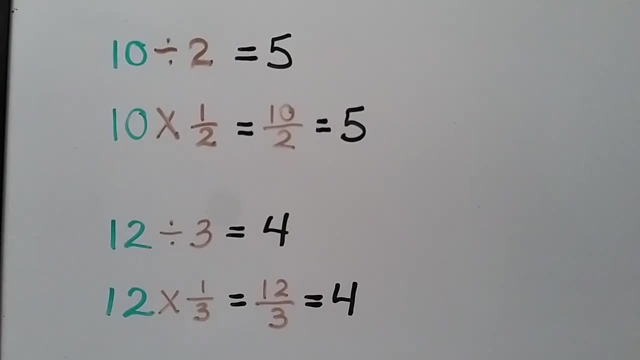 direction that the arrow is going. And remember: 10 divided by 2 is equal to 5.. We could also divide the first number by 4, plus one move and multiply it by one. do 10 times 1 half and that will be equal to 5.. 12 divided by 3 is equal to 4 and 12.